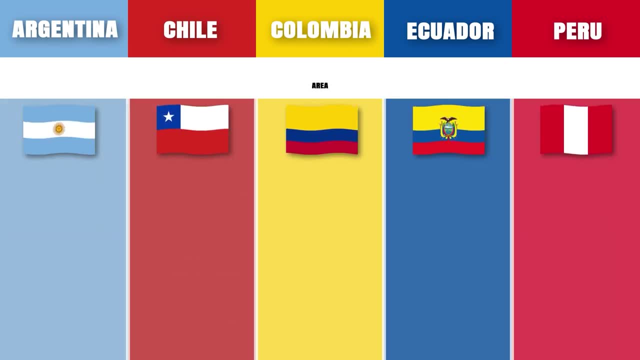 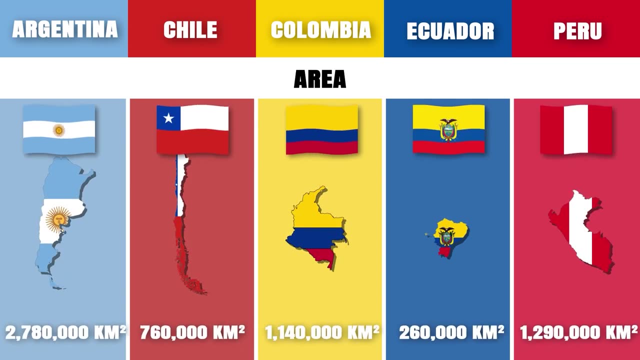 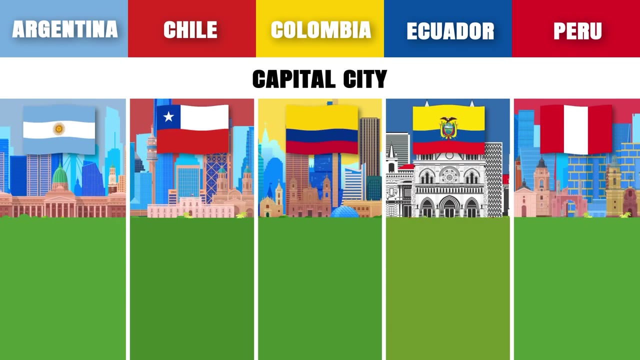 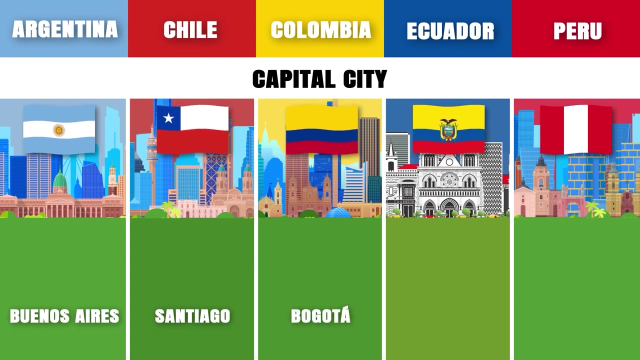 Peru Area. Argentina is the largest country, with an area of approximately 2,780,000 square kilometers. Capital City- Capital cities are Buenos Aires for Argentina, Santiago for Chile, Bogota for Colombia, Quito for Ecuador and Lima for Peru. 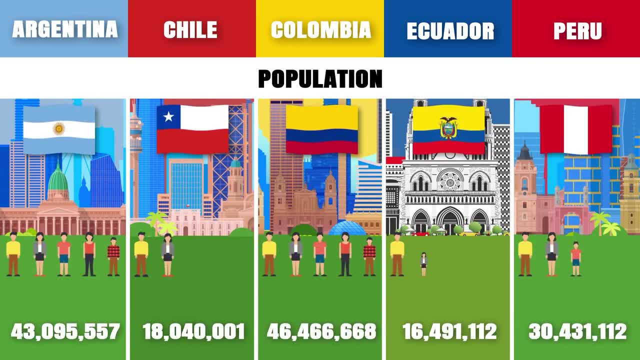 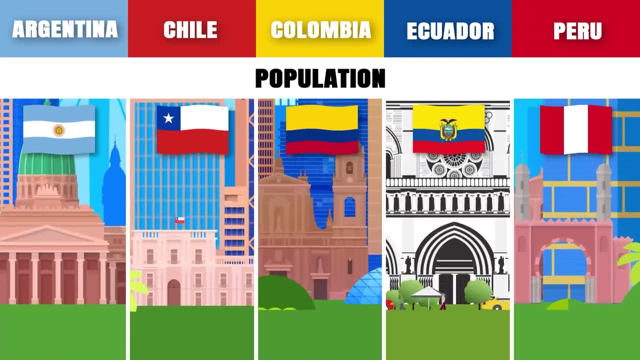 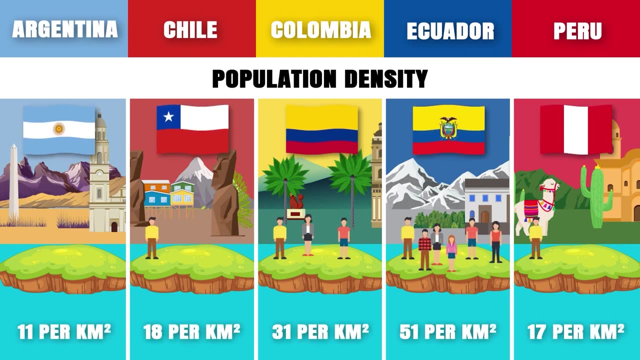 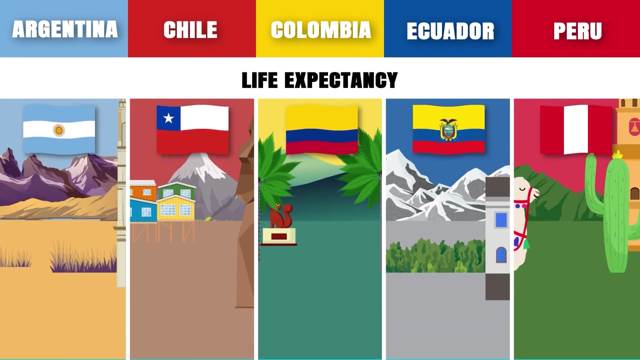 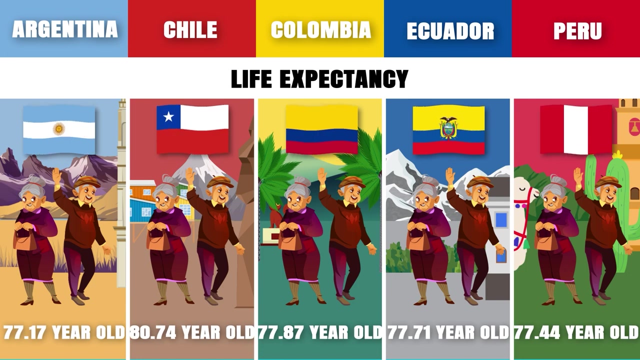 Population: Colombia is the most populous country, with about 51 million people. Population Density: Ecuador has the highest population density, with approximately 69 people per square kilometer. Life Expectancy: Chile has the highest average life expectancy, with a life expectancy of 80.7 for years. 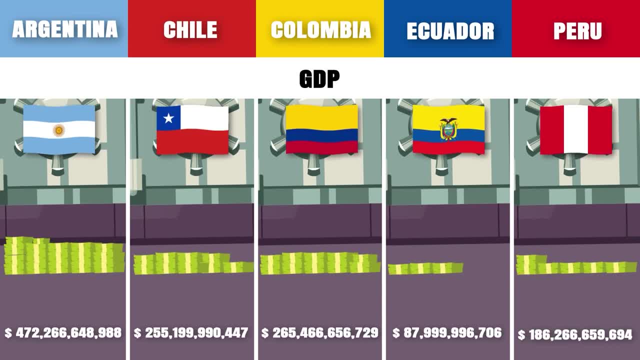 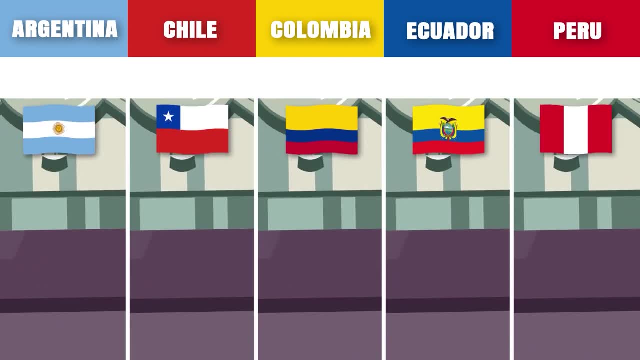 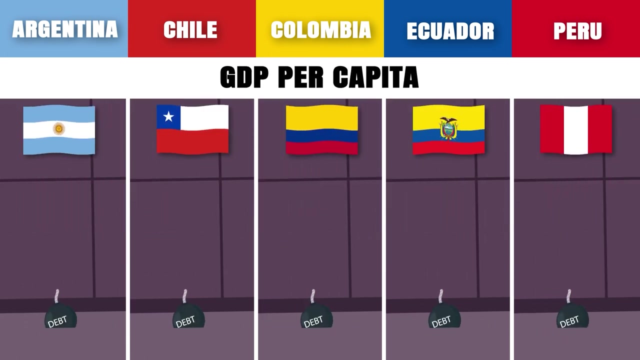 GDP: Argentina has the largest economy, with a GDP of approximately 644 billion US dollars. GDP Per Capita: Chile has the highest GDP per capita, with a GDP per capita of 17,280 US dollars. Debt-to-GDP Ratio: Argentina has the highest debt-to-GDP ratio. with approximately 69.5% of GDP. Export Chile had the highest export value, with a total export value of approximately $94,700,000.. Export Chile had the highest export value, with a total export value of approximately $94,700,000.. 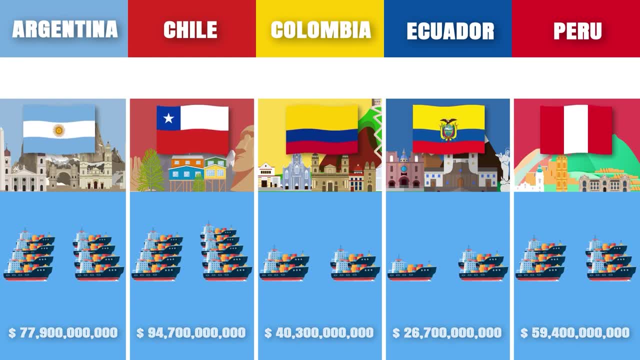 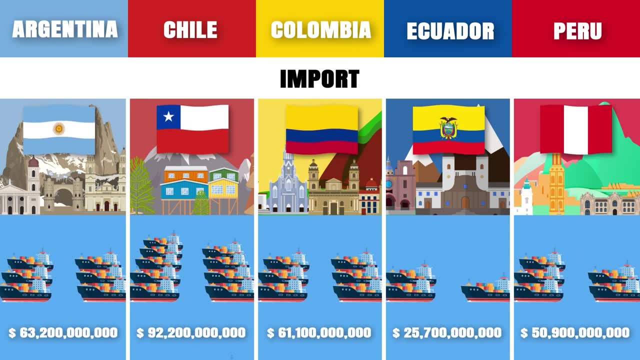 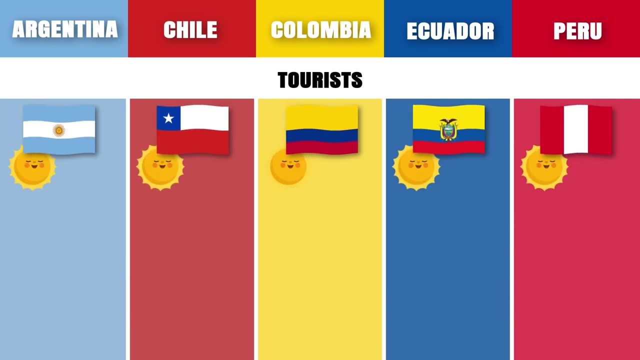 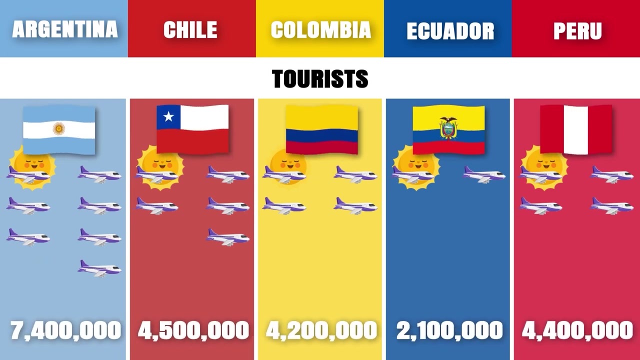 World Trade Festival, огод. Import: Chile also had the highest import value, with a total import value of approximately 92 billion to 100 million US dollars. Tourists: Argentina is the most visited country, with a total 7,400,000 tourists per year. 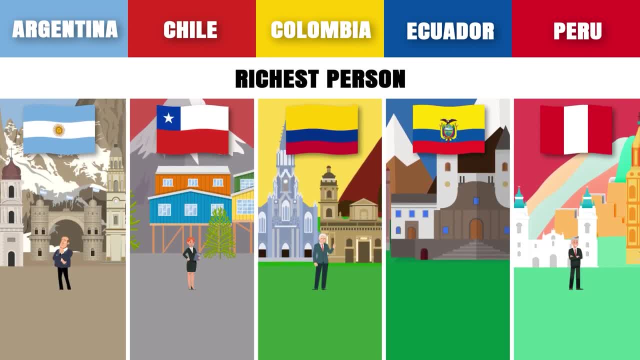 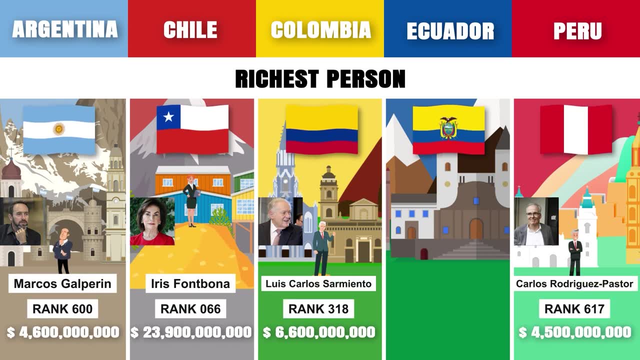 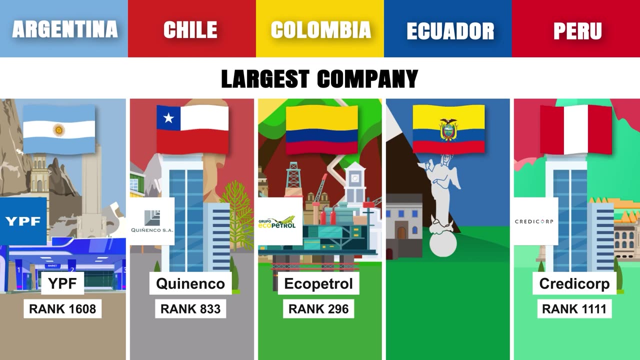 Francer longo: Mensch, delicious cookies. Richest person: Iris Fontbona is the richest person in Chile, with a net worth of approximately 23 billion 900 million US dollars. Largest company: Ecopetrol is the largest company in Colombia.